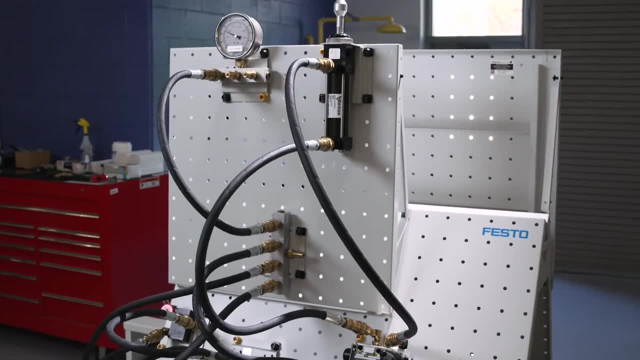 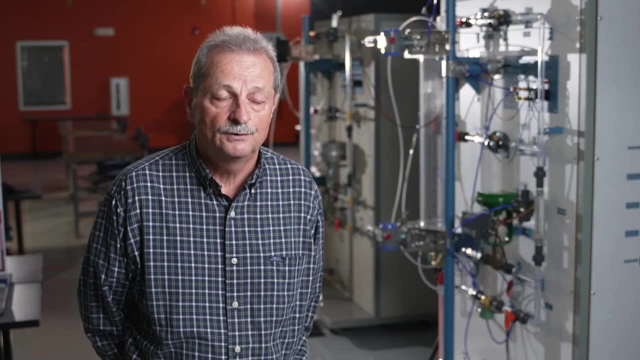 the robotic positions, what to do? We have the hydraulic trainer, the pneumatic trainer. Both of these are used in a lot of different types of industries. Also, we have electric motors and controls that the students receive hands-on to have an understanding of these. 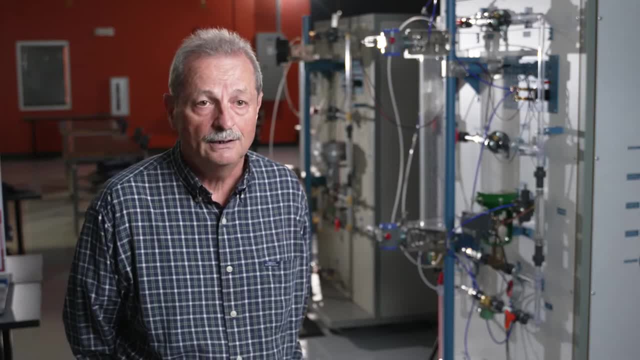 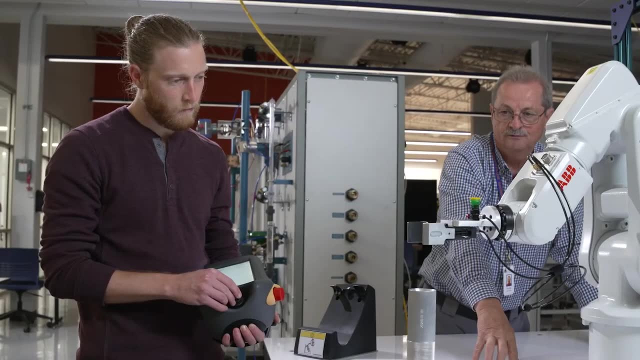 circuits so that when they do get a job and a career in that area they will know how to troubleshoot. and that's a big thing with the industries today. When I started in the mechatronics program I really knew nothing about it, but my instructors helped me to learn the equipment and 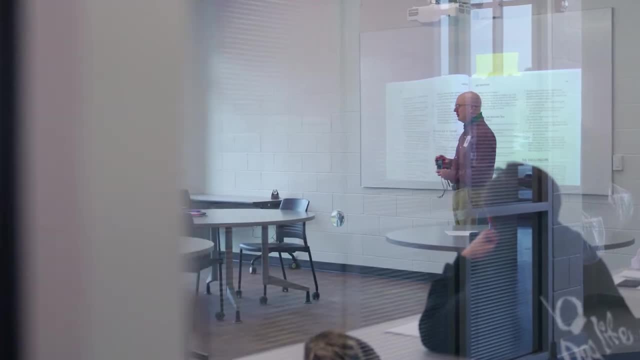 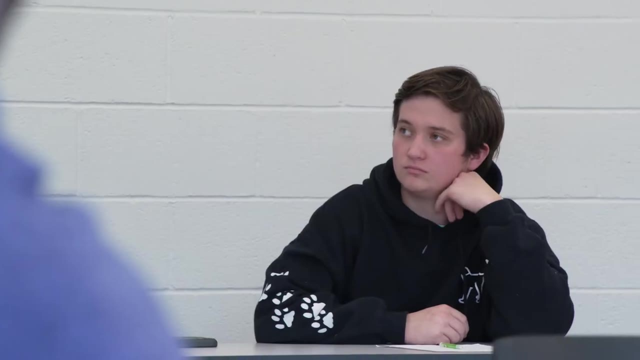 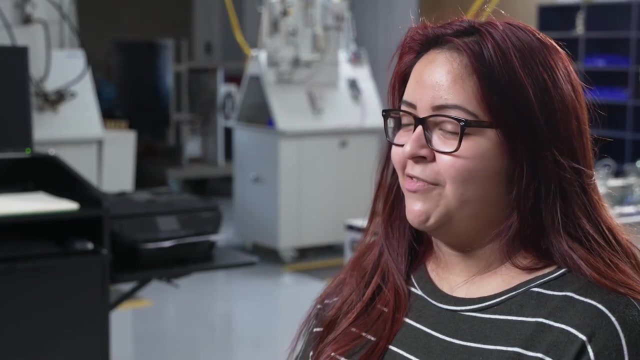 to get more interested in it. Small class sizes here at SCC allows the instructor more time to do more individualized training, which helps them to develop at a faster pace. I like that. it's really hands-on and I'm a really hands-on person. I really cannot just read out of a book. 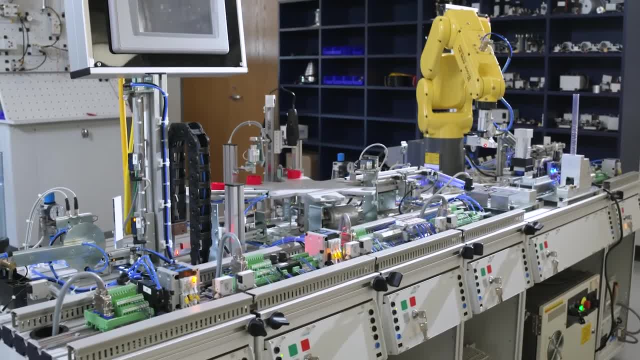 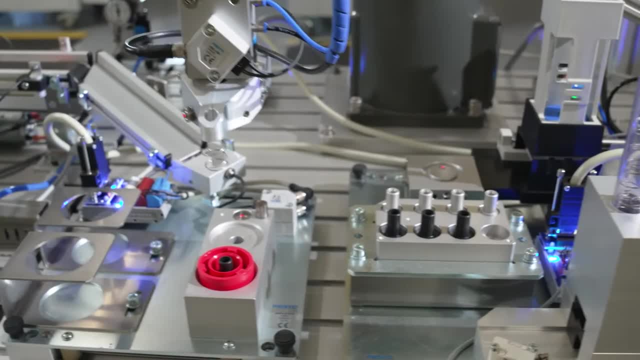 Through the coursework that you'll be involved with. we have a mechatronics trainer using a robotic arm to assemble four parts together. It gives them a first-hand look at the advanced manufacturing out in the industry. The equipment here at Southeastern. it's really advanced. 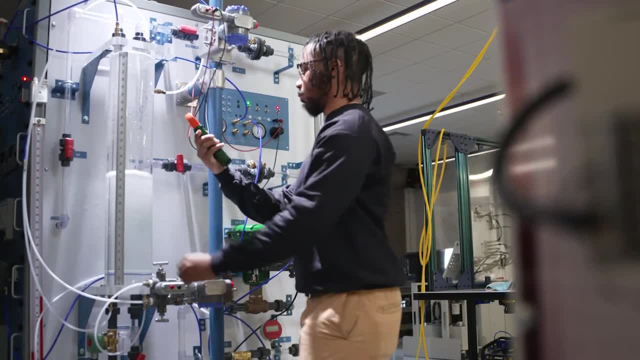 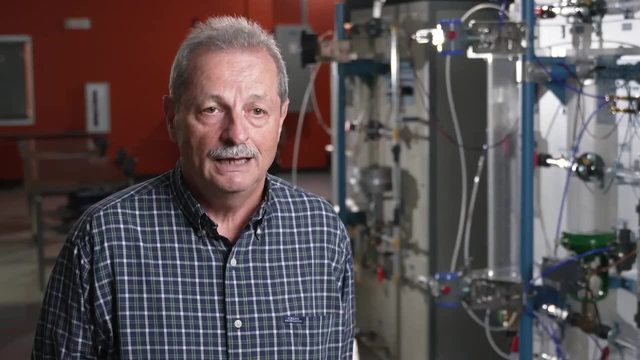 It's really interesting because it has a lot of the components that most facilities outside of Southeastern will have. Many careers require both mechanical and electrical disciplines and when you have both of those you are a much better fit for the industries what they're. 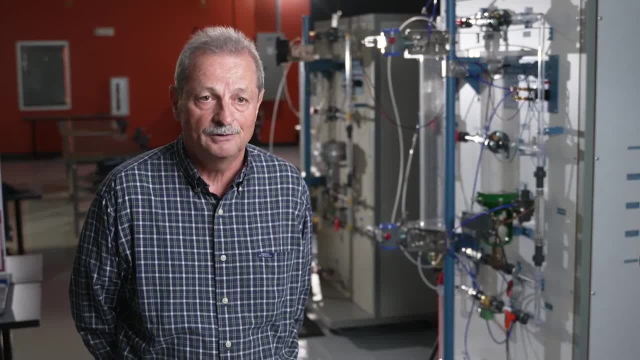 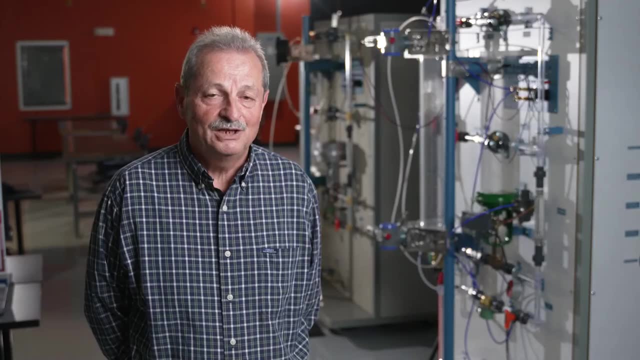 looking for. Therefore, you have a long-time career with that type of industry. After I graduate from Southeastern, I plan on going to the automobile industry and working with their automated systems. Many students with a two-year degree here at SCC in the subject of mechatronics they will go. 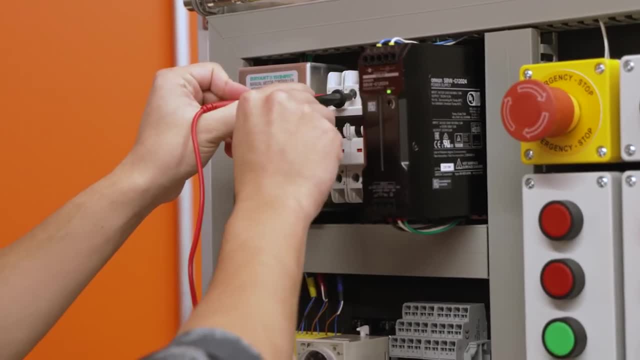 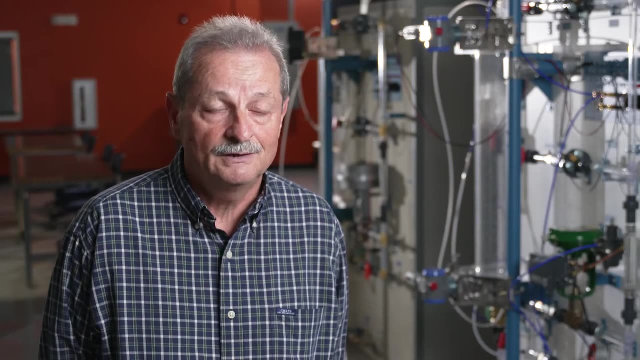 straight to the workforce. Others will have the opportunity to go, maybe, to a four-year university. We have a transfer to East Carolina, a bachelor of science in industrial technology, which many of those will go on and receive. that, What I would say to someone wanting to learn more? 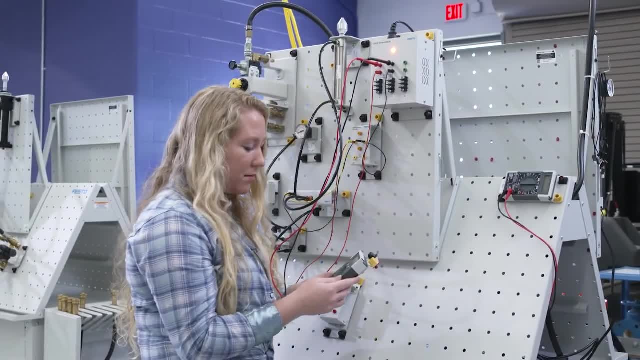 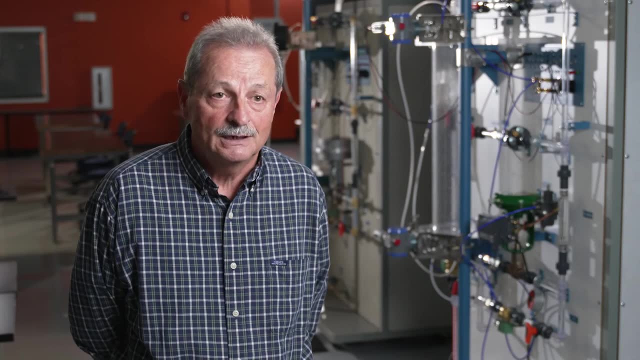 about mechatronics is: try a website inside the Eastern Community College or try contacting an instructor to help you understand a little more about it. Any of you that would like to contact us here at the college feel free to. If you have any questions, we'll be glad to.